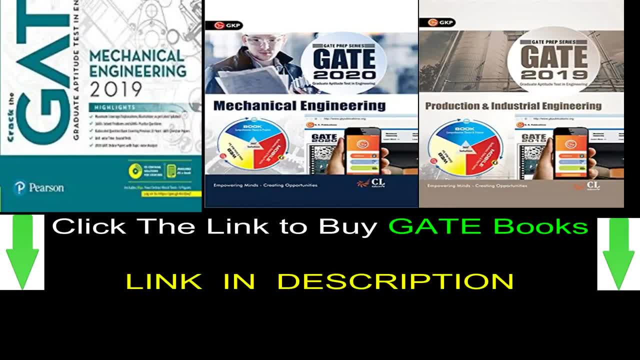 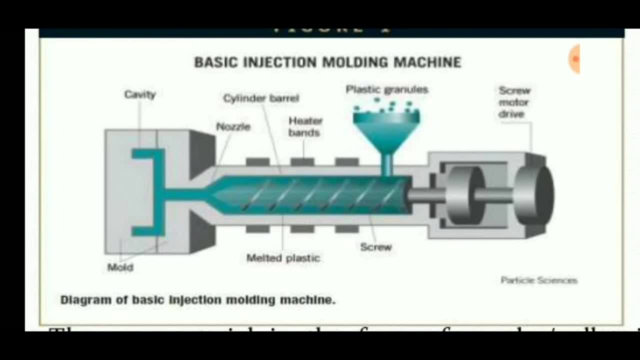 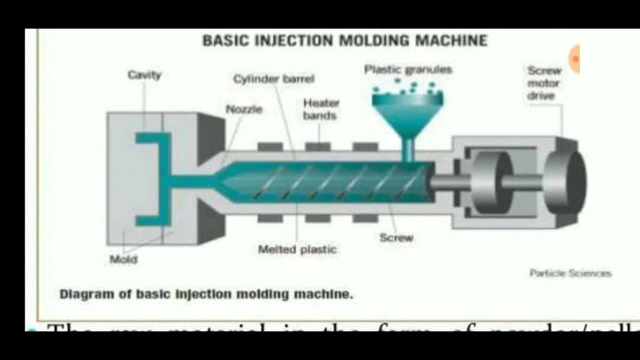 Hello viewers, welcome to engineering study materials. Today we are going to discuss about the injection molding process, So let's get into this video. In this process, plastic granules are inserted inside the hopper and it consists of a heated cylindrical component surrounded with the heaters so that the plunger is used to push the plastic granules through the heated chamber where the plastic granules are inserted. 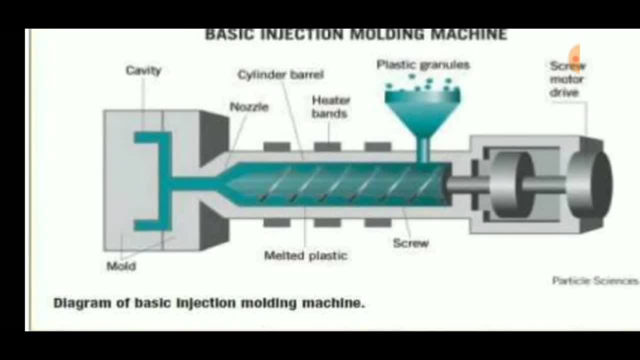 It melts to a liquid state and then, with the help of the mixers, it is forced to inject into the cavity of the molds. The molds consist of a: one is a fixed mold, another is a movable mold. Finally, it cures, and then the part can be taken out. 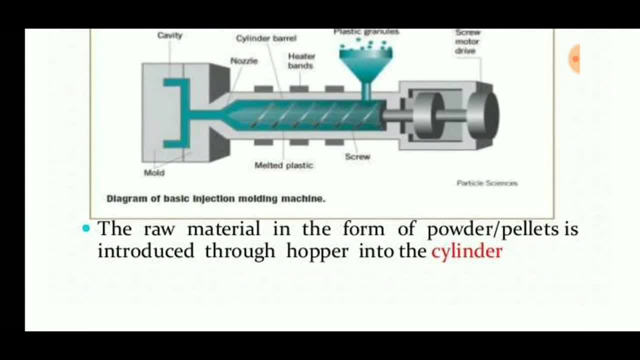 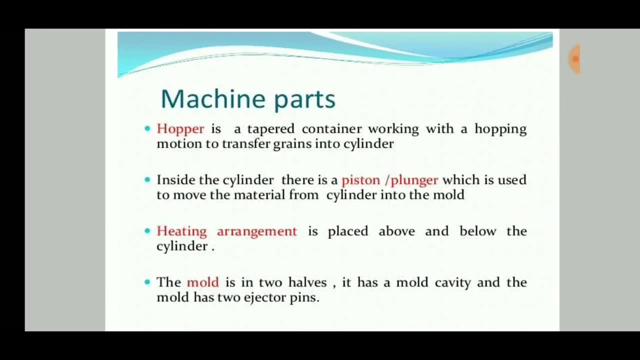 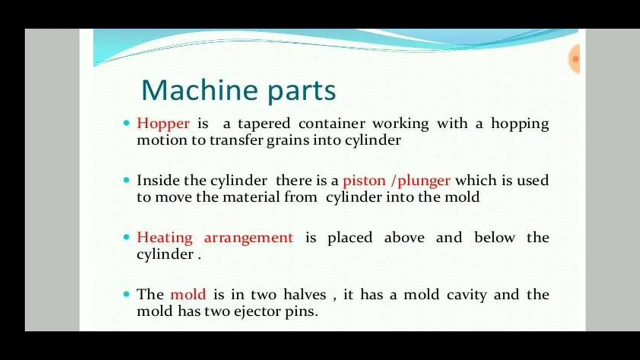 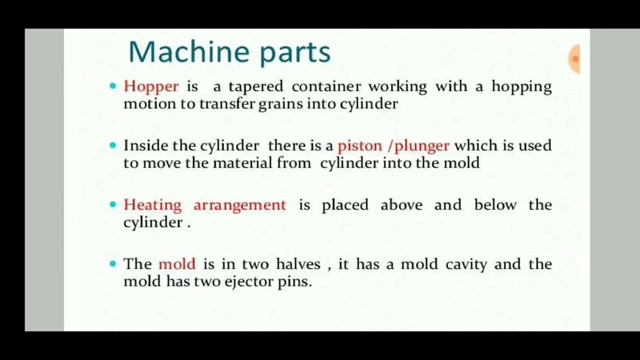 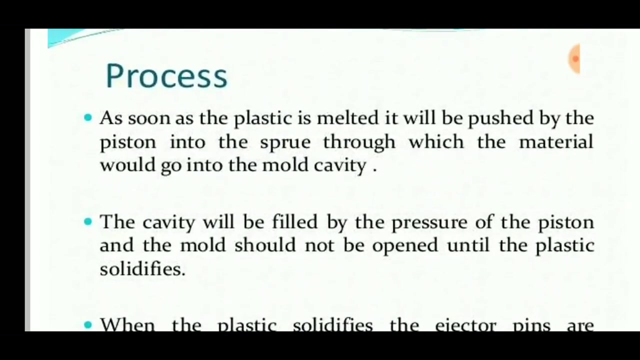 This procedure are: the raw material in the form of a powder or a pellet is introduced to the hopper. The hopper is placed through the hopper into the cylinder. then it is the hopper is a tapper container. inside the cylinder there is a plunger or a piston which is used to move the material from the cylinder into the mold and a heating arrangement is placed above and below the cylinder. The mold consists of two halves. It is made as a mold cavity and molds has the two ejector pins and as soon as the plastic is melted it is pushed by the piston into the sprue. 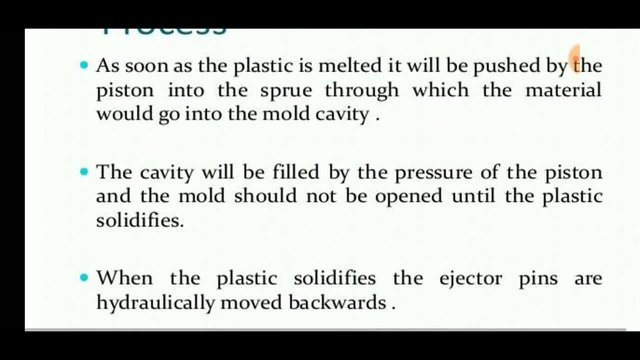 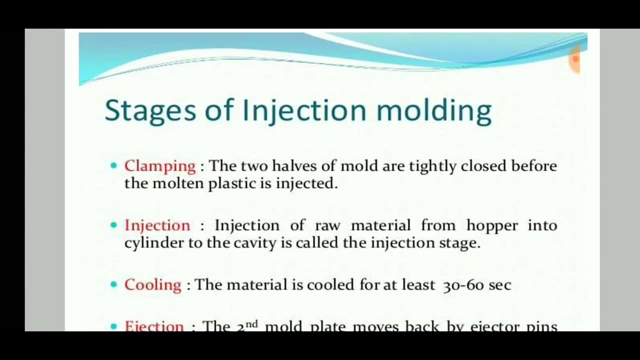 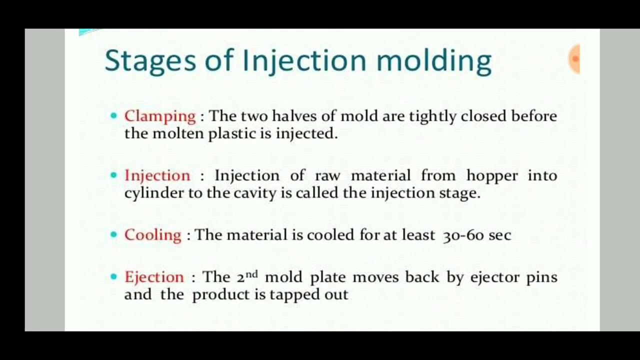 Through which the material would go into the mold cavity. The cavity is allowed to cool so that the plastic can be able to solidify. Finally, the part can be taken out. There are some stages of the injection. molding are clamping, that is, two halves are the mold are tightly closed injection: injection of the plastic, then cooling: the plastic cools to. 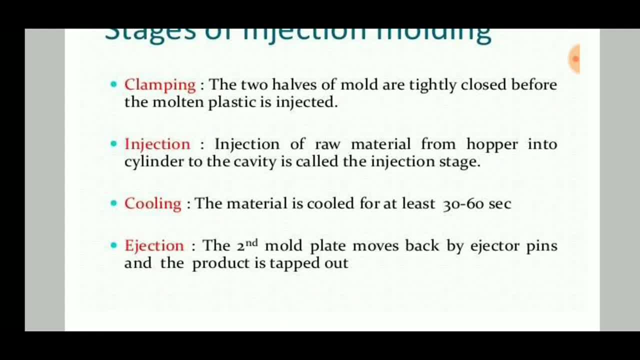 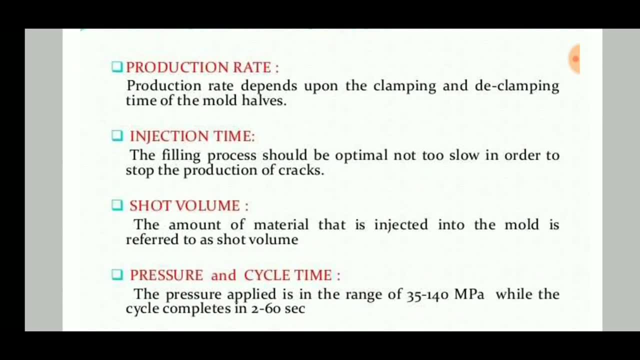 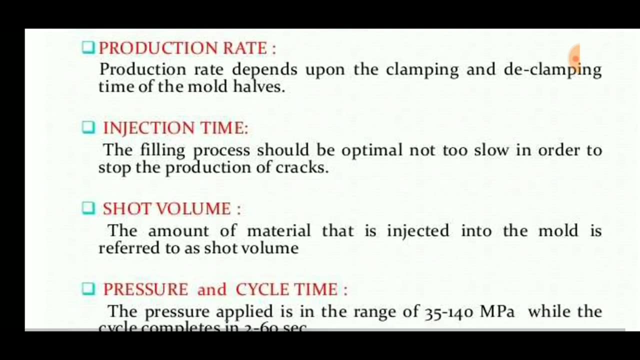 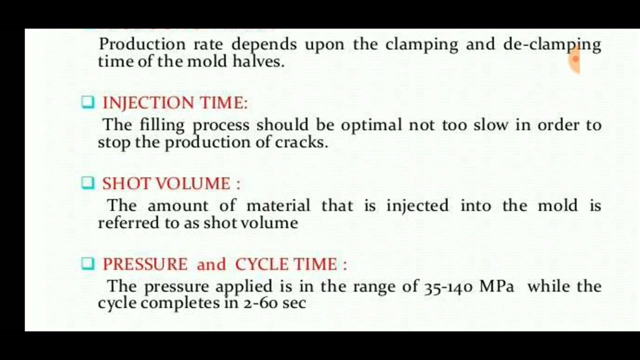 go into the solidified state, then injection: the solidified part is taken out. the important applications are characteristics of: the production rate is high. it is based upon the clamping and decamping time and injecting time, the filling process for the plastic into the cavity, then short volume, the amount of material that is injected, and pressure and cycle time. high pressure causes the molten metal to solidify.